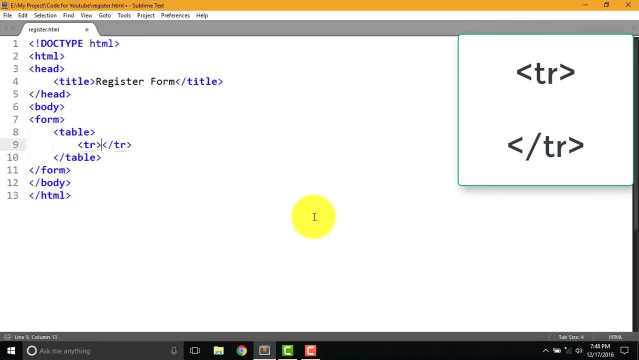 Create first row with tr and td for table data where we put name and input field. Now, first I'm gonna write name Again, type td, Then type a following code: angle bracket: input type equal to text. Again type tr for password field, Then type td. 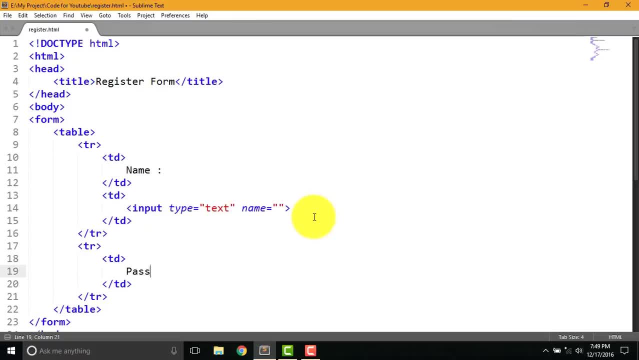 And password Type td again for input field of password. Now write following code: input type equal to password. Let's see how it's done Here. you can see this form only contain name and password. Let's type some additional code for input box. 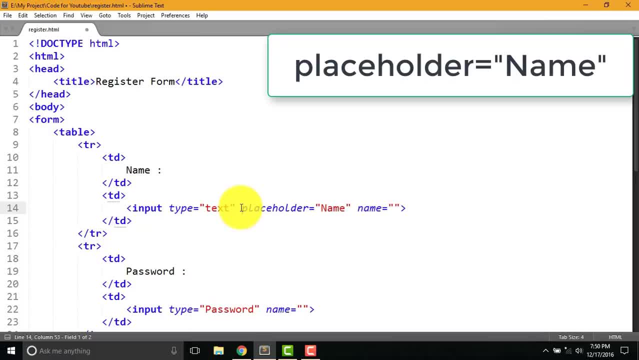 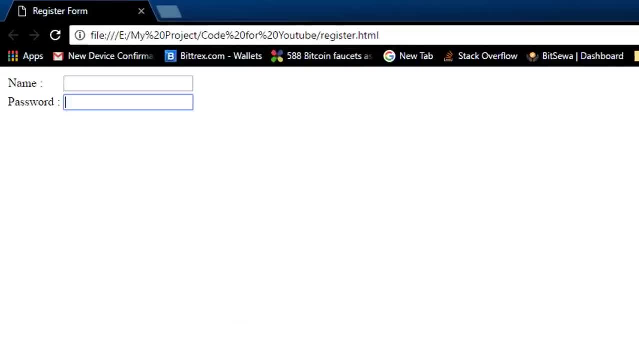 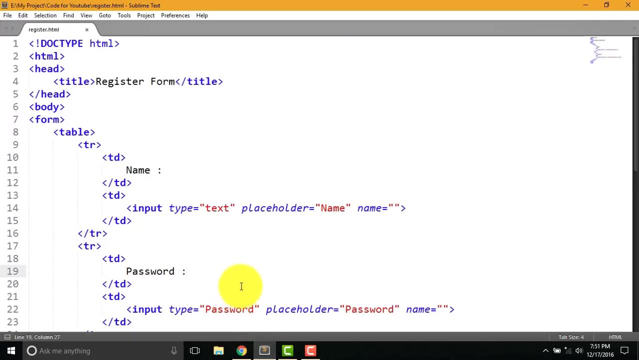 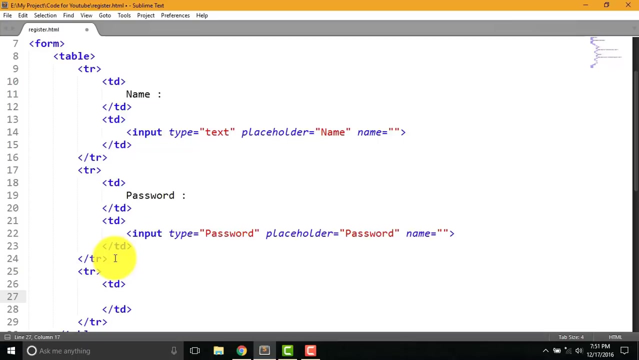 Type: placeholder equal to name. For password field placeholder equal to password. Here you can see the changes. after adding a placeholder code, Now add a code for gender. For that we have to write tr and td again, Then write gender. Create another td to choose male or female. 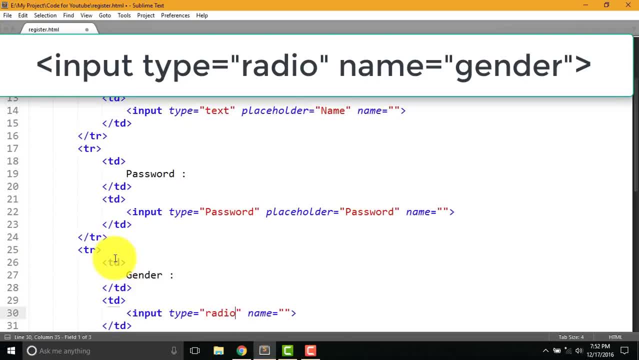 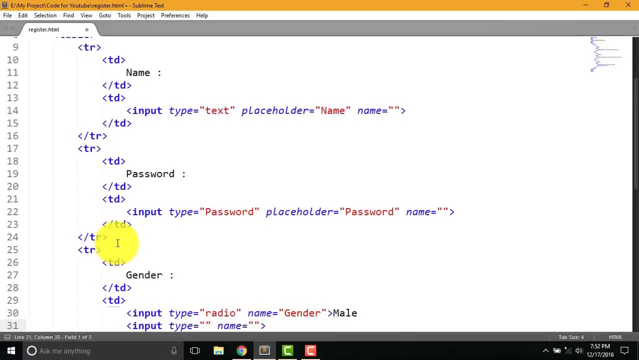 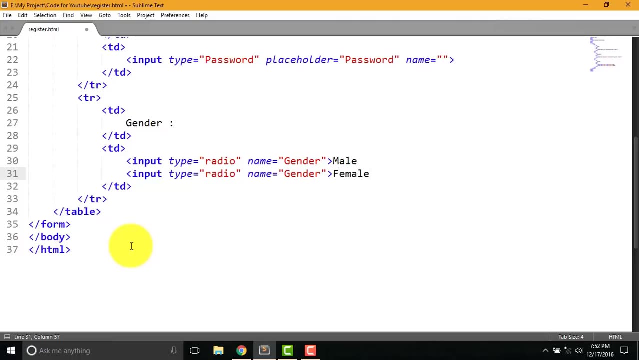 Write input type equal to radio and name equal to gender. After that type male, Then type same code for female also. After that type tr and td again for email. Now type email, Then type td and write following code: Let's see how it's done. 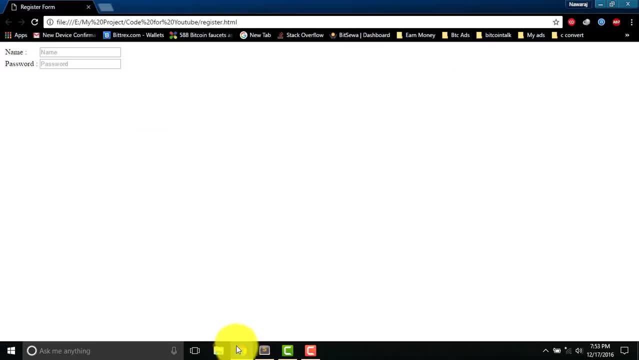 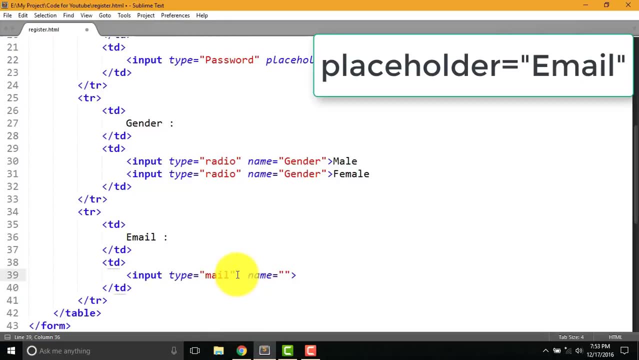 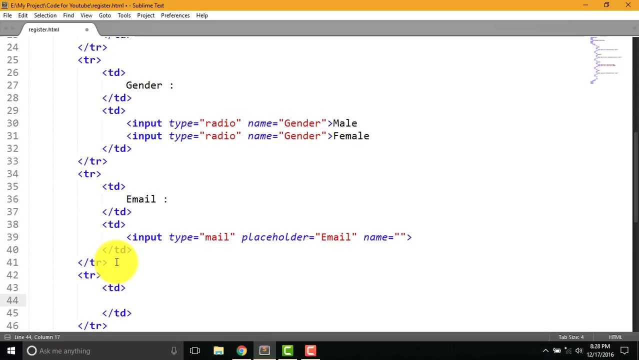 Let's see how it's done. Why forget placeholder for email? Just write placeholder equal to email. Now it look little better. Now write tr and td For phone number. After that I'm gonna write td for the list of country code.